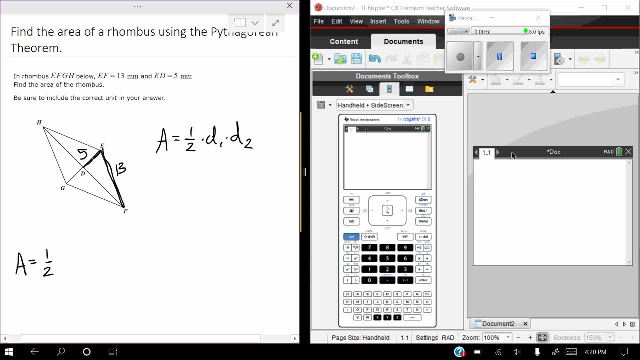 The first would be here, this distance from E to D. So the distance from E to D is 5, so the distance all the way across from E to G would be 10.. So that's diagonal 1, we'll call it 10.. 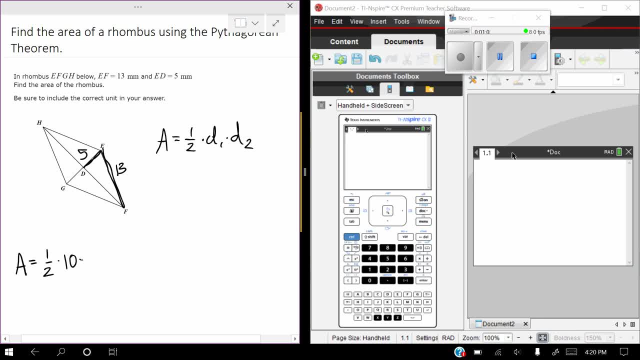 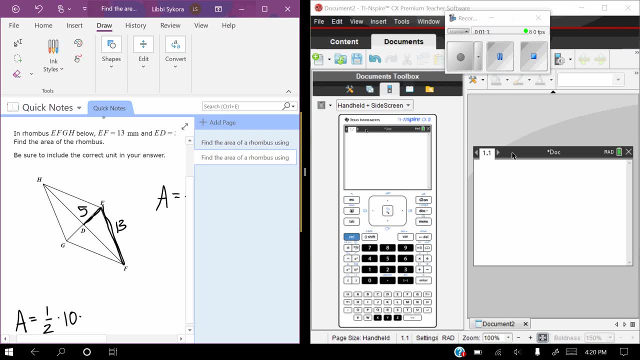 We need to find diagonal 2. And before we can do that, what we have to do is figure out the distance from D to F, And what you need to remember for this is that in a rhombus, the diagonals meet at a right angle. 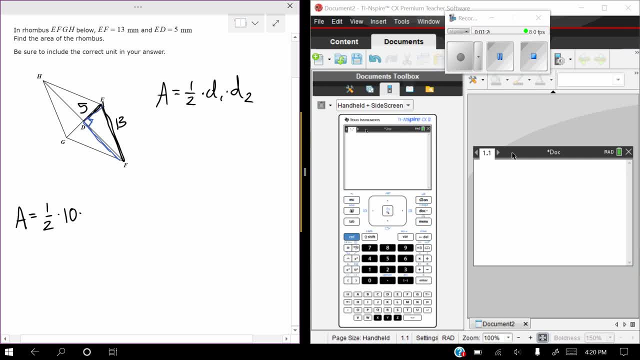 So I know that right here I'm looking at a right triangle. So I'm going to do this, This Pythagorean theorem, because if I have a right triangle and two sides, and then I'm looking for the third side, that's what we're going to use. 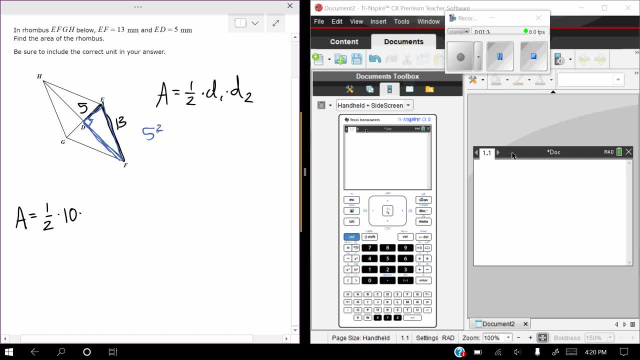 So we're going to go a squared 5 squared plus. we'll call this x plus x squared equals 13 squared. I want to just remind you really quickly: 13 is the one that goes by itself because it's the hypotenuse. 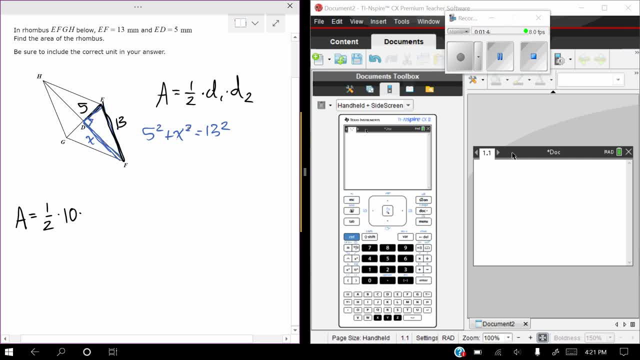 The hypotenuse is always the side across from the right angle, and that's the one that goes by itself. So we've got: 5 squared is 25, plus x squared Equals 13 squared, which I think is 169,. yep. 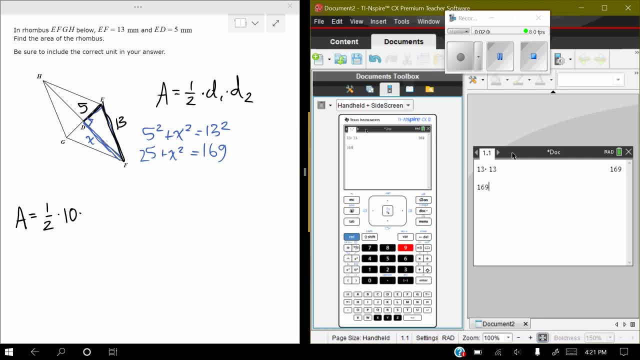 So we've got 169 minus 25.. So x squared equals 144.. We'll square root both sides of that and x will equal 12.. So I know the distance from here to here is 12.. But I need to figure out what's diagonal too. 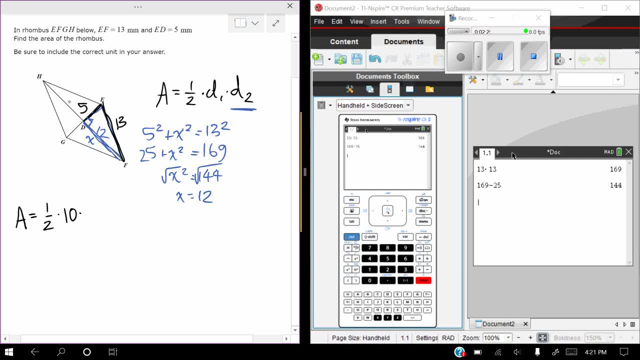 That's what I really want to know, And I know that 12 is only going to be half of this diagonal, So the whole distance from f to h is going to be 24.. Oops, 24.. So that's going to be my what I type in the calculator: 1 half times 10 times 24, 120. 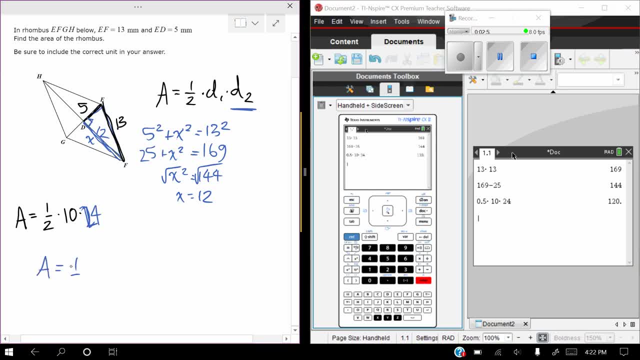 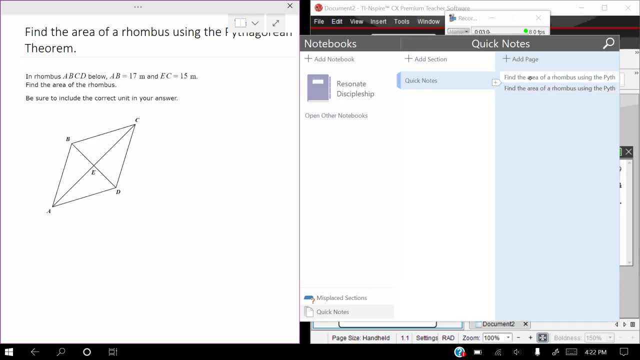 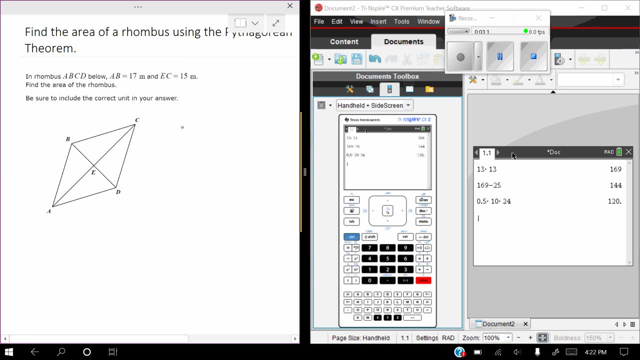 That's what we're looking at. Let's try one more together. And the rhombus abcd below ab is 17.. So the distance from a to b is 17. And the distance from e to c is 15.. And the distance from e to c is 15.. 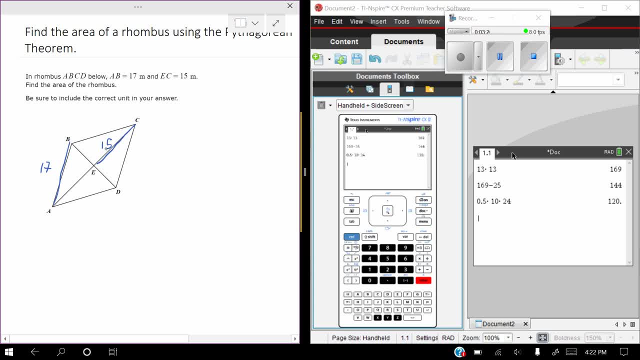 And the distance from e to c is 15.. We need to find the area of the rhombus and be sure to include the correct unit in our answer, While you're looking at this and you're like, wow, those sides don't even touch. 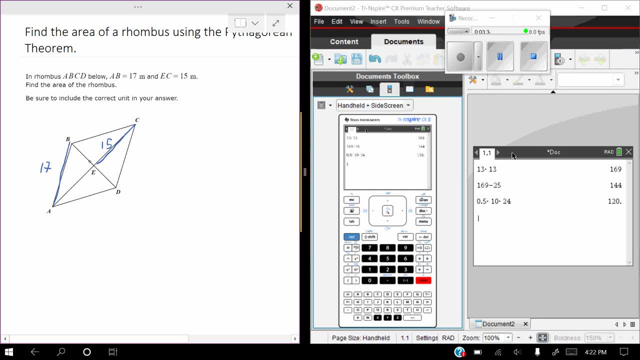 But what I do know is that in a rhombus diagonals bisect each other, So this side also is going to be 15.. Okay, So in this quest to find area of a rhombus, 1 half times diagonal, 1 times diagonal, 2,. 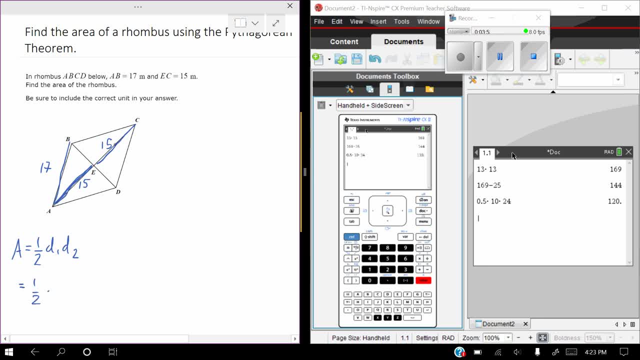 I'm going to go 1 half times diagonal: 1. from a to c is 30, and now i just gotta find diagonal too. so, remembering, in a rhombus, diagonals are perpendicular. they meet at a right angle. i'm going to solve this right triangle. 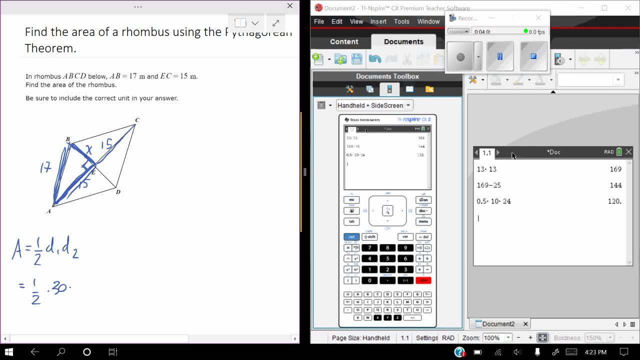 right here. i'll call this side x with the pythagorean theorem. so we've got x squared plus 15 squared equals 17 squared. okay, so i'm going to just subtract 15 squared from each side. this would be maybe a quicker way to do this. 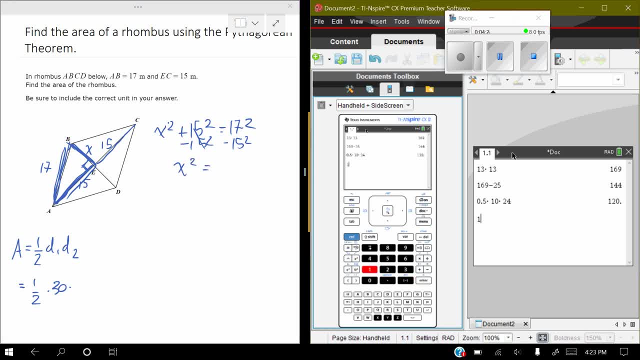 so we've got x squared equals 64.. so then x would equal 8 when you square root both sides. so this is 8 right here, which means the entire diagonal from b to d. that entire diagonal is going to be 16. so that's going to be, when i type in my calculator, one half. 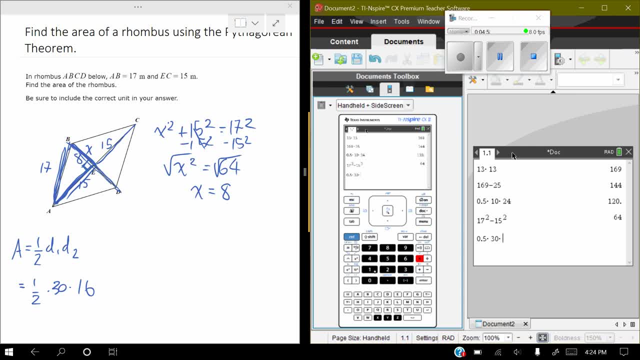 times 30 times 16. 240 and that will be in meters squared. and that's your answer. that is how you find the area of a rhombus using the pythagorean theorem.